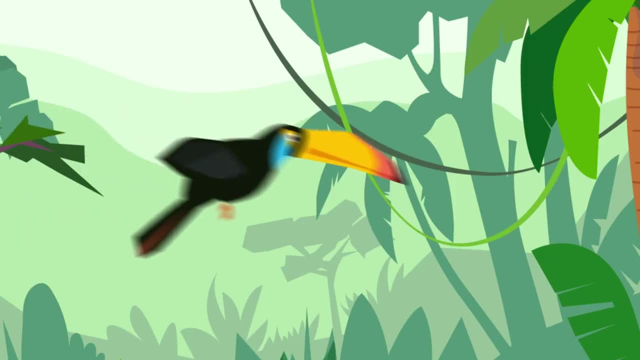 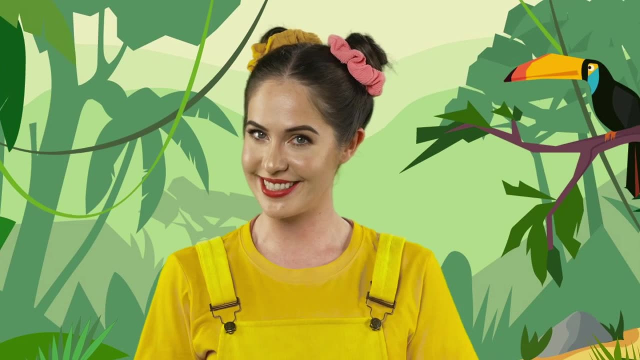 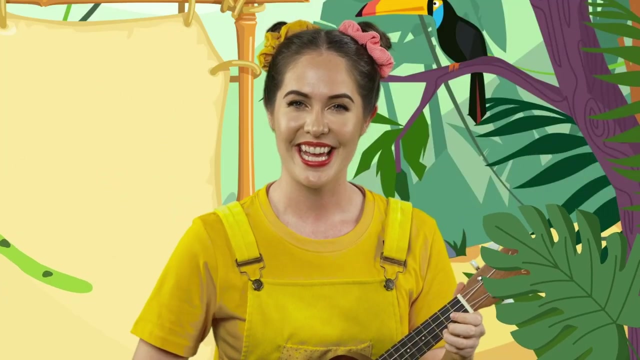 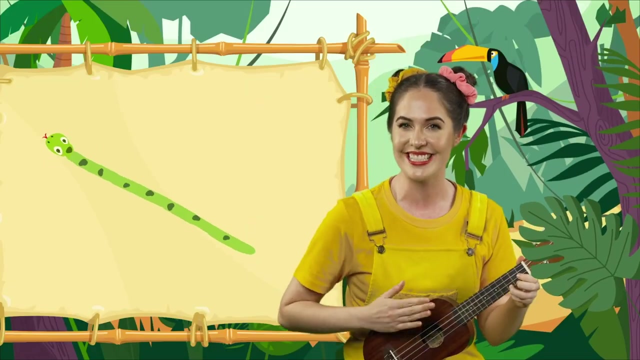 My friend Sammy the Snake can twist and bend into some super silly shapes. Let's use our voices and our fingers to trace Sammy, Sammy. Sammy, Sammy the Snake, Get your finger ready to trace the shape he makes. Sammy, Sammy, Sammy the Snake, Get your finger ready to trace the shape he makes. 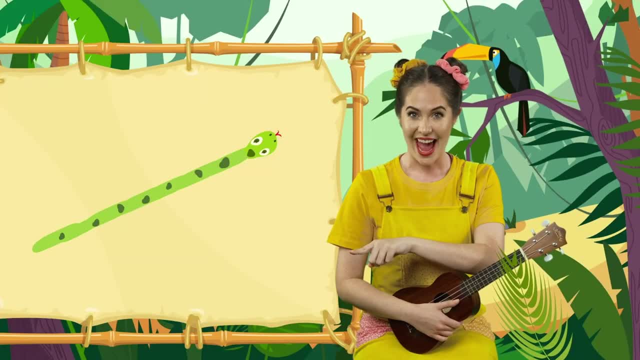 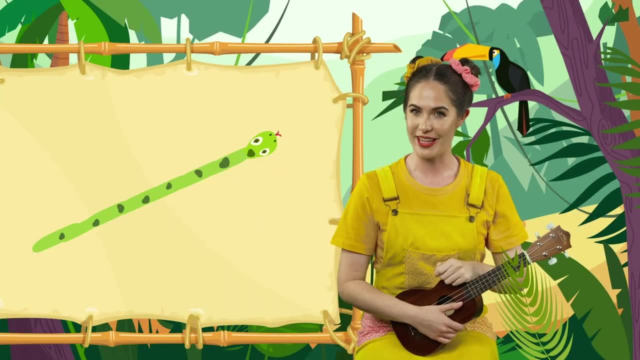 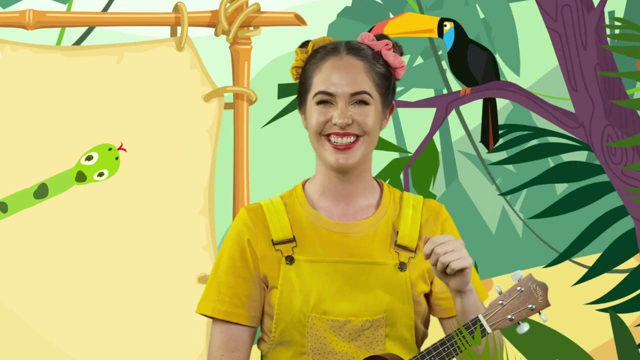 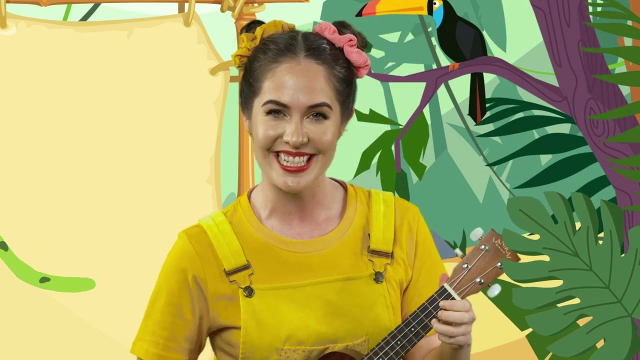 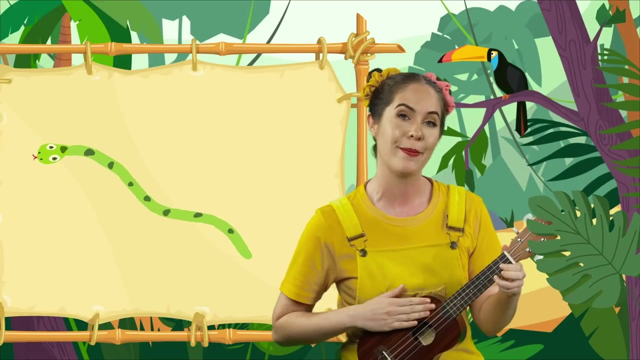 He starts down low and stretches up high. We can start down low with our voices and stretch up high. Great job, Sammy, Sammy, Sammy the Snake. Get your finger ready to trace the shape he makes. Sammy Sammy, Sammy the Snake, Get your finger ready to trace the shape he makes. 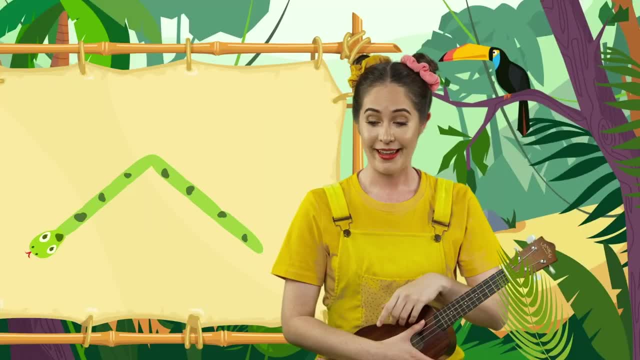 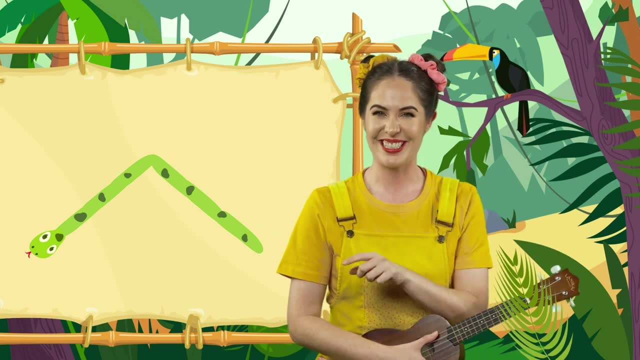 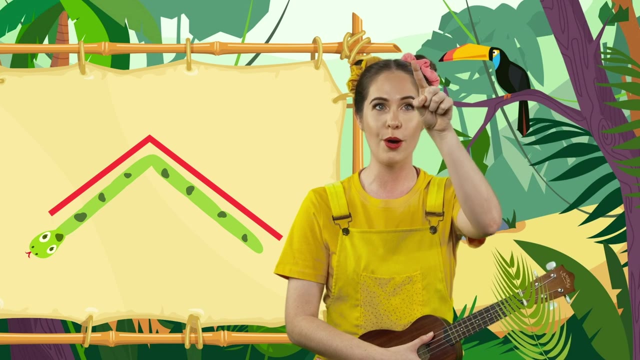 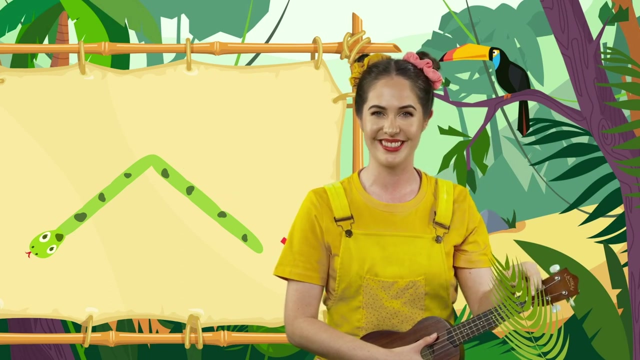 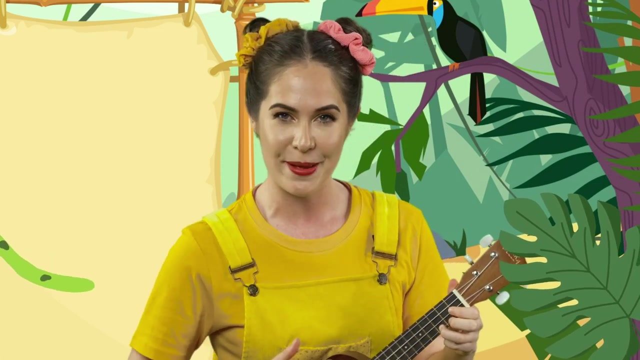 Sammy has a big bend in his body. He starts down low, He stretches up high and comes back down. Sammy has a big bend in his body. He stretches up high and comes back down low again. Let's have one more. go, Sammy, Sammy, Sammy the Snake, Get your finger ready to trace the shape he makes. 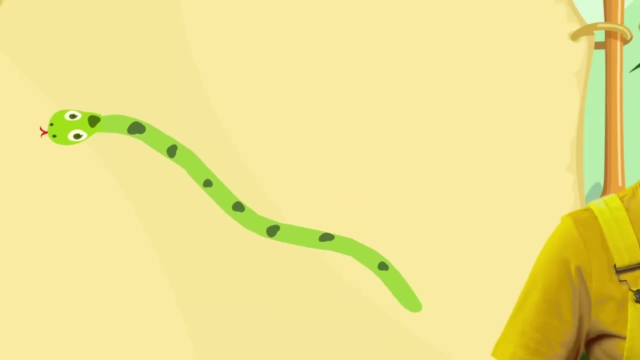 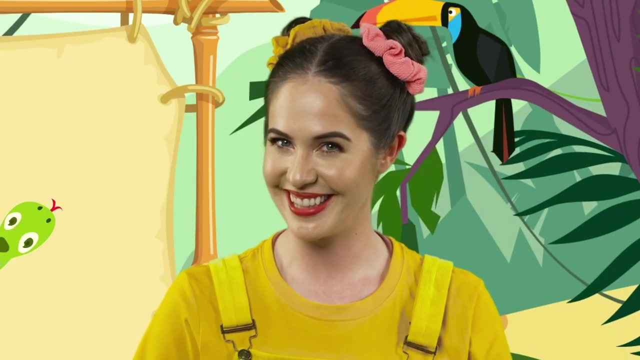 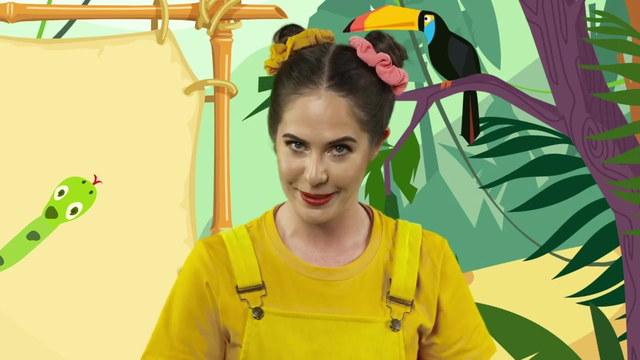 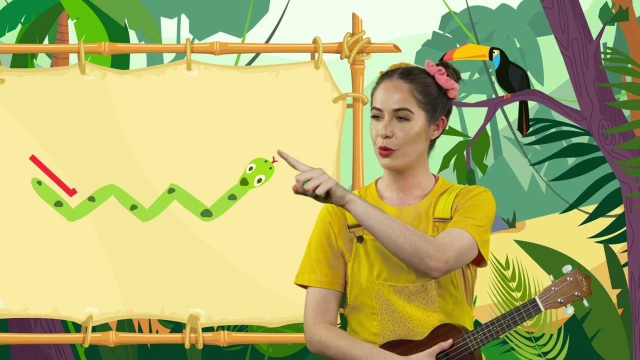 Sammy, Sammy, Sammy the Snake, Get your finger ready to trace the shape he makes. This is a silly one. Sammy is very bendy. He goes down and up, and down and up. Let's have a turn together One more time. 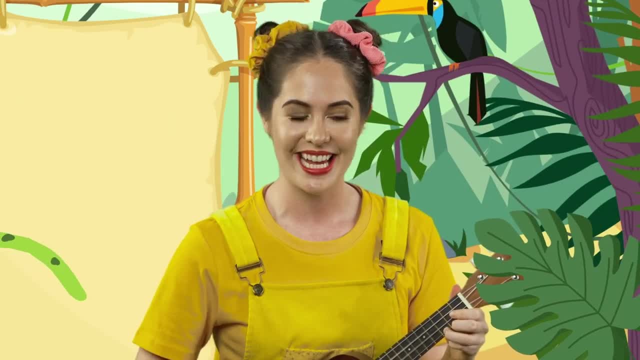 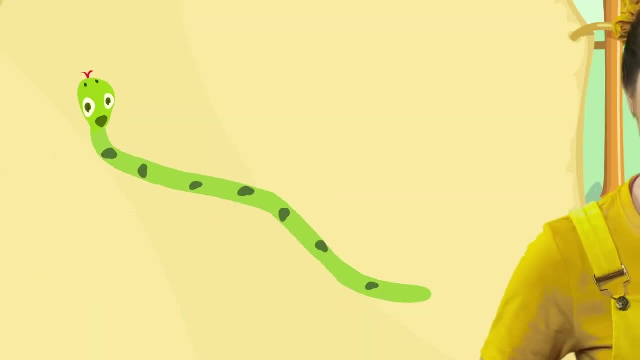 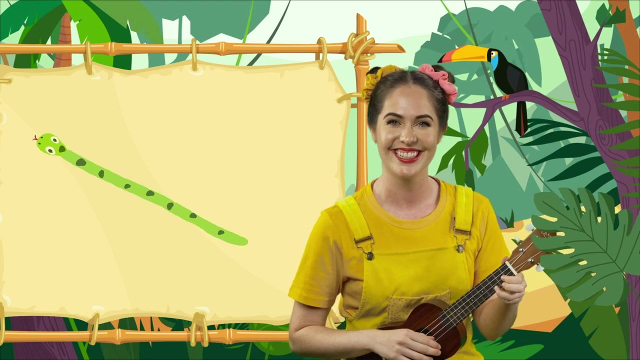 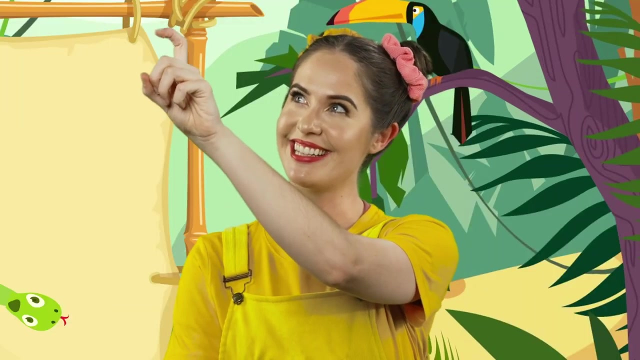 Well done, Sammy, Sammy, Sammy the snake. Get your finger ready to trace the shape he makes. Sammy, Sammy, Sammy the snake, Get your finger ready to trace the shape he makes. Start with your finger up high. He starts up high and goes down low.